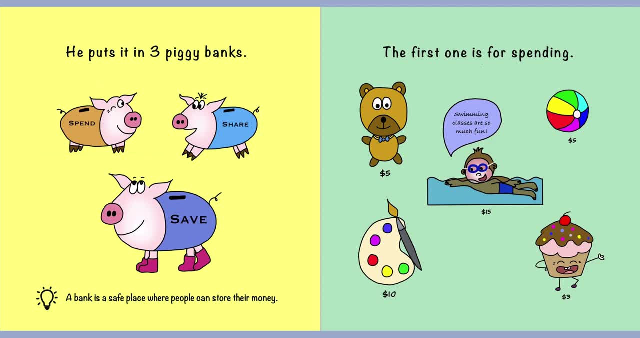 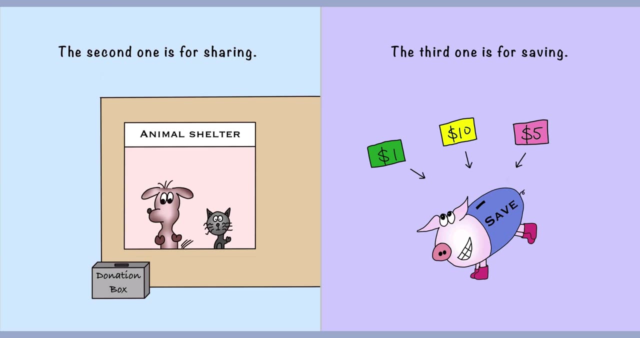 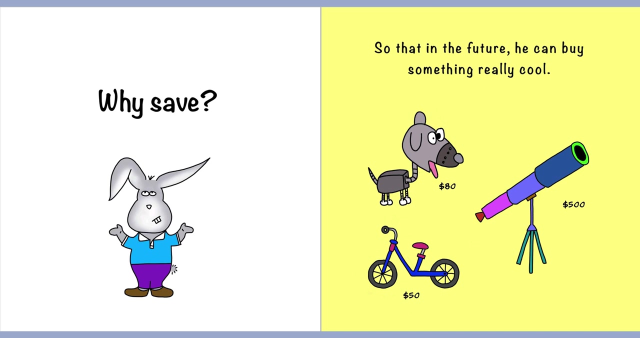 A bank is a safe place where people can store their money. The first one is for spending: Swimming classes are so much fun. The second one is for sharing. The third one is for saving. Why save? So that in the future he can buy something really cool. 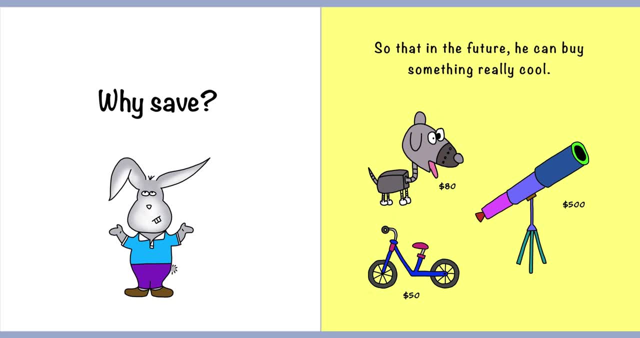 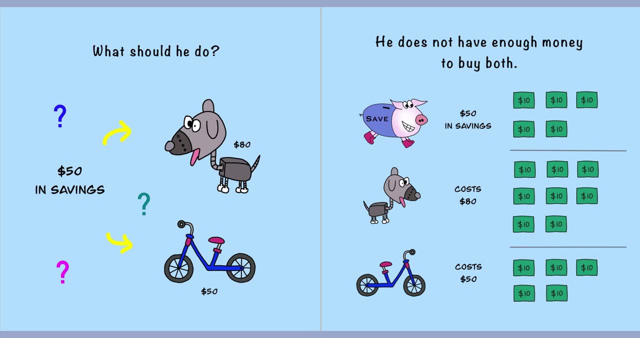 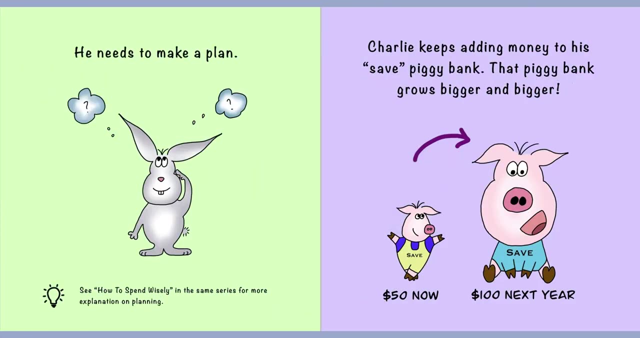 What should he do? He does not have enough money to buy both. He needs to make a plan. See how to spend wisely in the same series for more explanation on planning. Charlie keeps adding money to his save piggy bank. That piggy bank grows bigger and bigger. 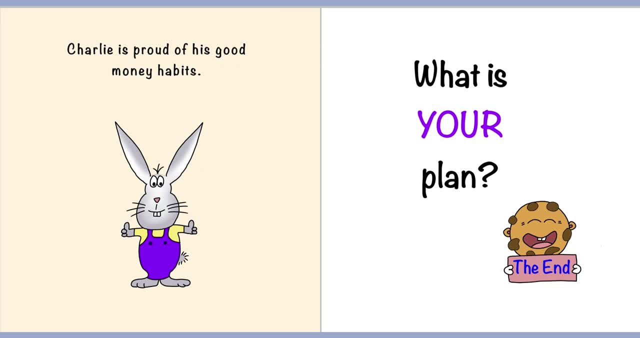 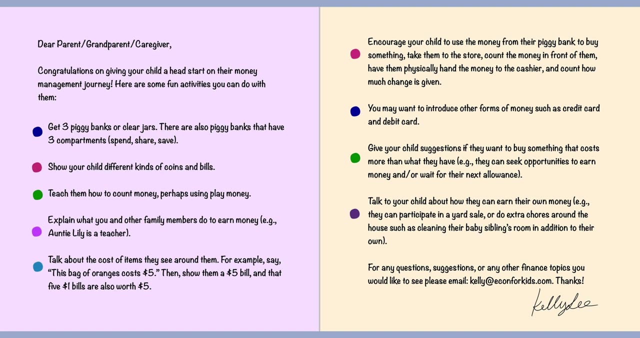 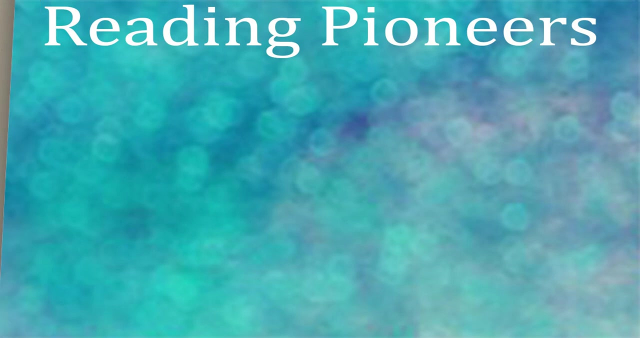 Charlie is proud of his good money habits. What is your plan? The end? Dear parent, grandparent, caregiver, Congratulations on giving your child a head start on their money management journey. Here are some fun activities you can do with them. Thank you, Pioneers, for reading with us today to the book What is Money by Kelly Lee. 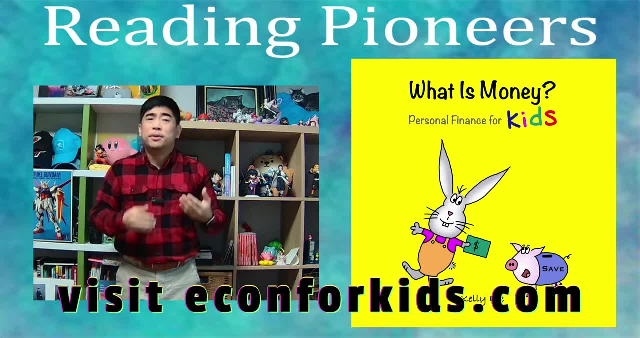 I loved reading this book because I think it's vital for children to grow up learning about finance and saving. My parents always told me to save, but now, looking back, I wish I saved more. If you enjoyed this book as much as I did, you can support Kelly by visiting her website, econ4kidscom. 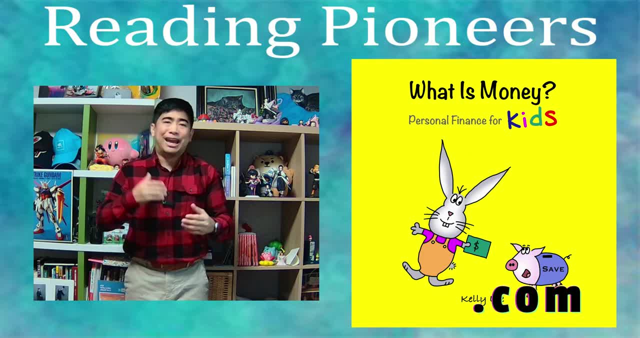 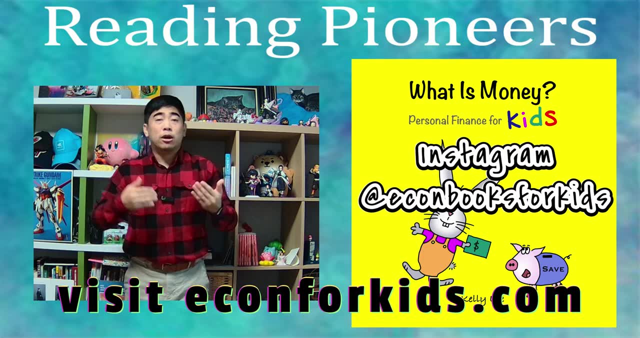 which has other great books dedicated to informing and teaching children about money and finance. Additionally, this book is available on Amazon as a Kindle ebook, hardcover and paperback, so I hope you do show some support in one of these ways. Links to all of them are available in the description. 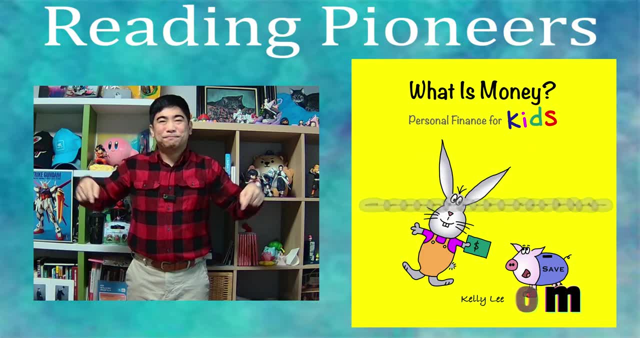 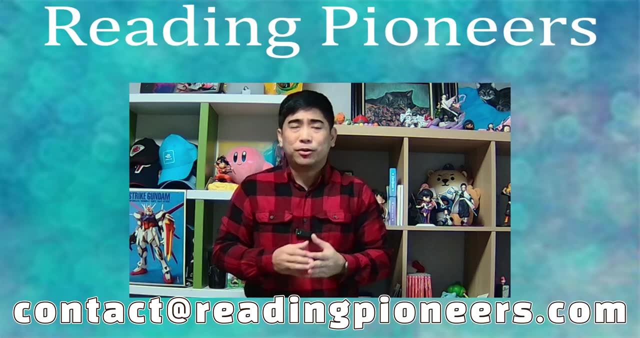 I'm so grateful that Kelly contacted me to read this book with you today. If you have a book you'd like to be read on this channel, please send me an email- contact at readingpioneerscom, so we can turn it into the next video.